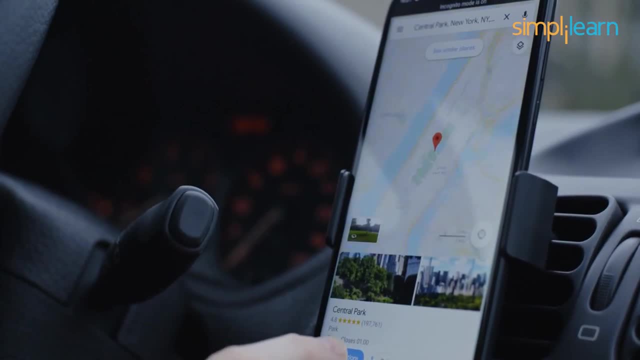 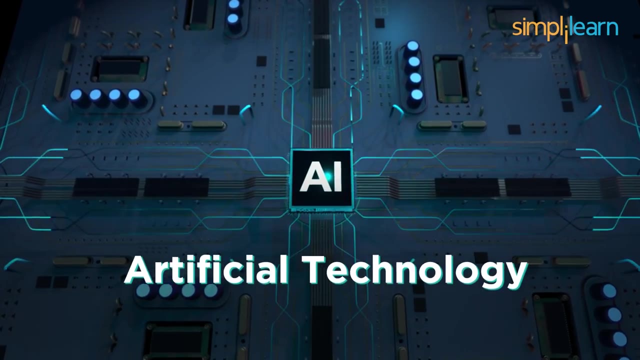 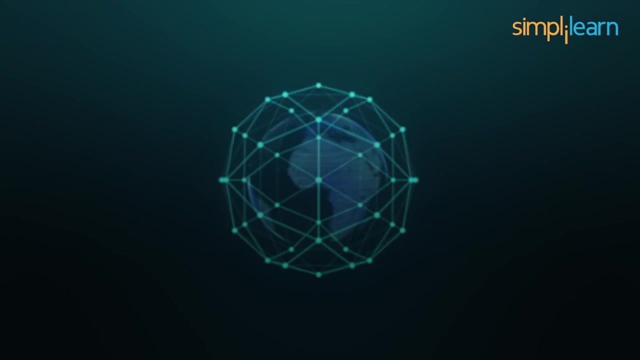 Ever wondered how Google Maps can provide the fastest route almost instantly? Have you ever considered the speed and accuracy of virtual bots like Google Assistant or Siri? All of them are powered by artificial technology- AI for short Riding on the data science hype train. the global AI market is projected to go from around $87. 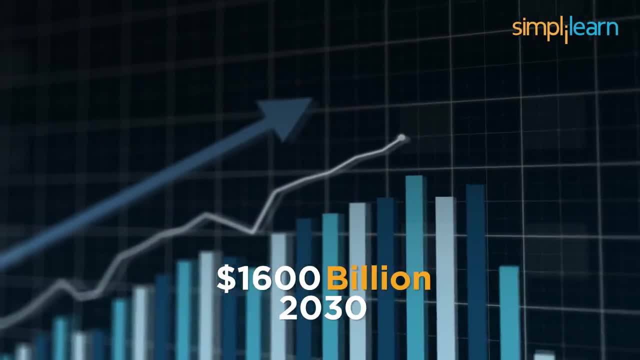 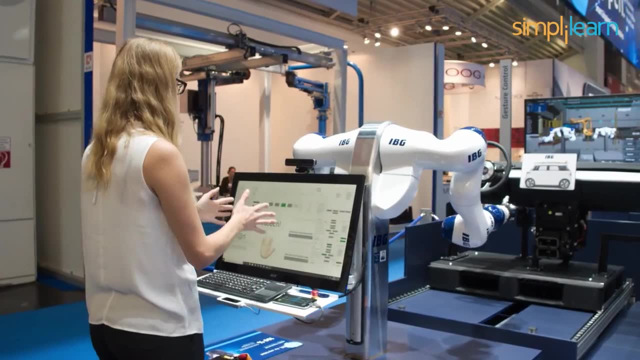 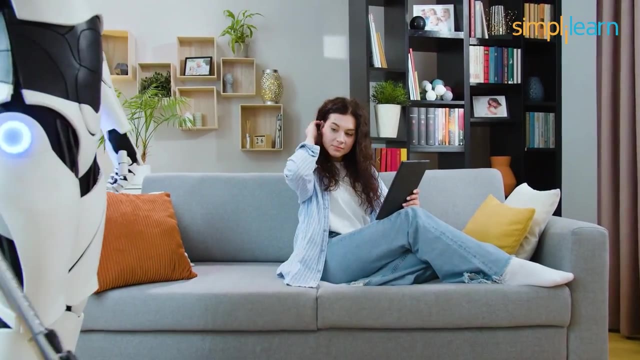 billion in 2021 to nearly $1600 billion by 2030.. Artificial intelligence has impacted almost all sectors of the IT domain, but its significance in the robotics industry is unmatched. Even Tesla has announced a new humanoid robot named Optimus, recently built to perform daily activities and help in Tesla factories. 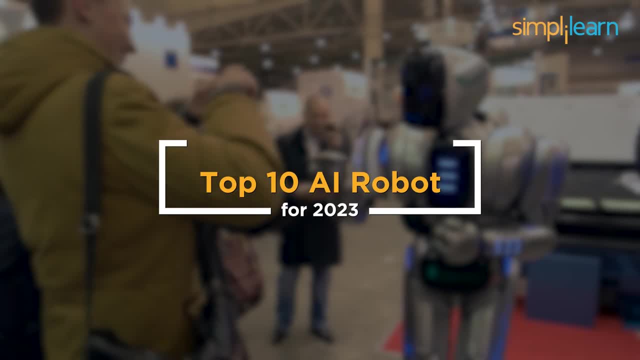 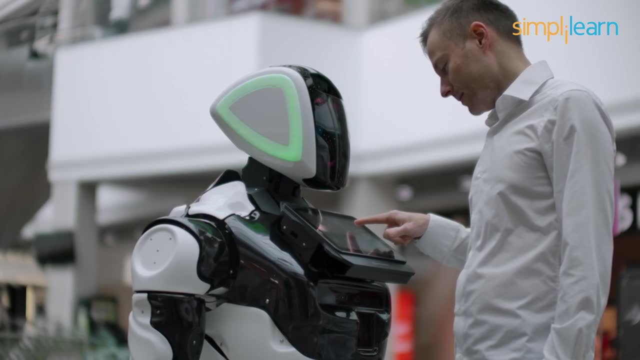 In today's video, let's go through some of the most advanced artificial intelligence-based robots, paving the way for a faster and smarter future in 2023.. Before we start, here's a question for the AI enthusiasts watching this video. Which one of the following is not an example of AI? 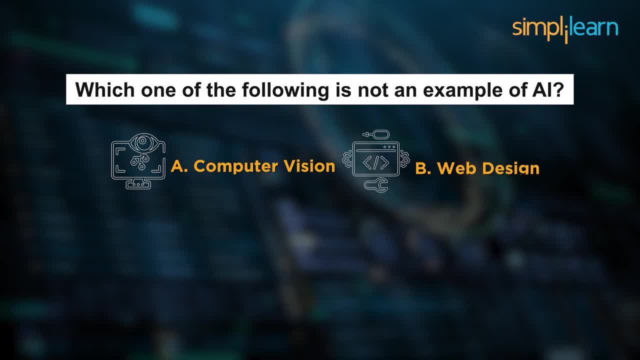 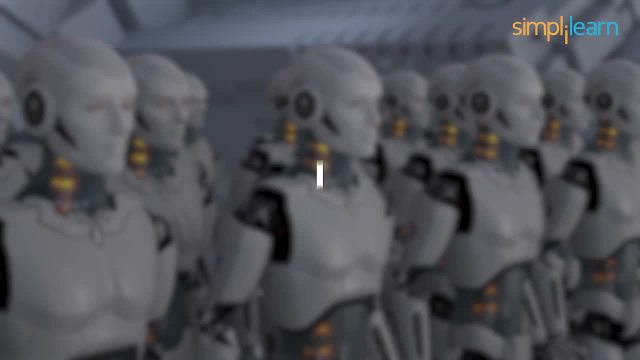 A- Computer Vision, B- Web Design, C- Voice Recognition, D- Robotic. Please leave your answers in the comments below, And that's our cue to get started with the Top 10 AI Robots for 2023.. Number 10 on our list is AIBO. 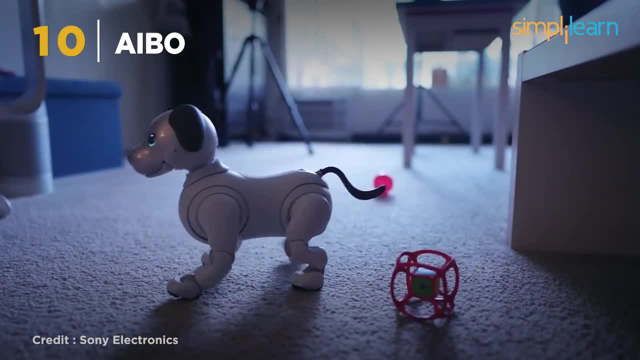 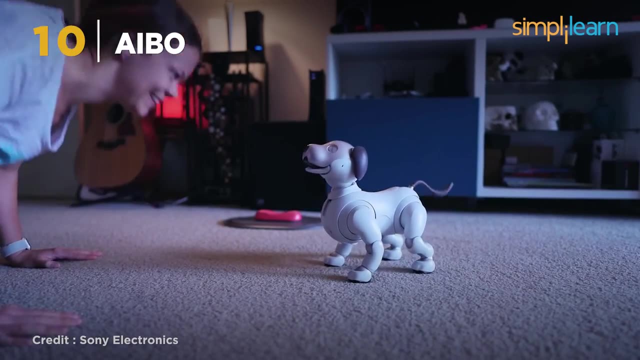 AIBO is a charming little robot dog created by Sony. This robot was retired nearly a decade ago but has been brought back with even greater human operation capabilities. This artificial puppy responds to words of praise or head scratches, can learn tricks and seeks out owners. 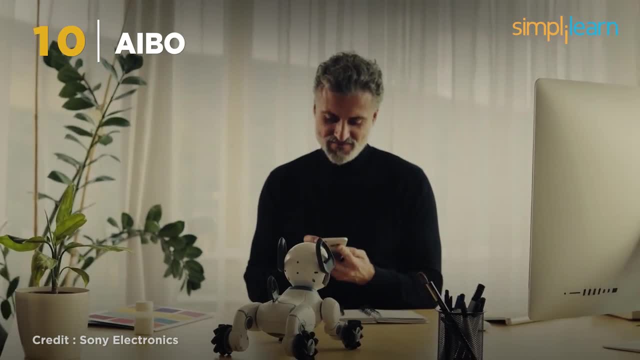 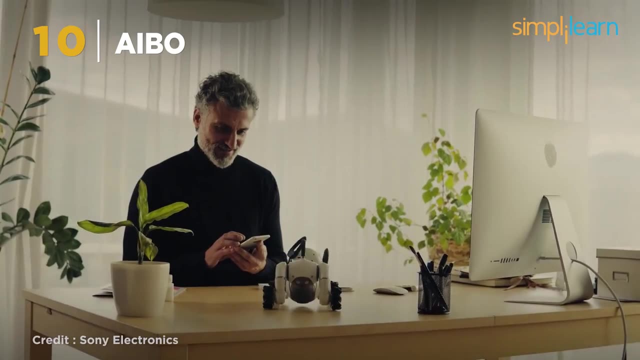 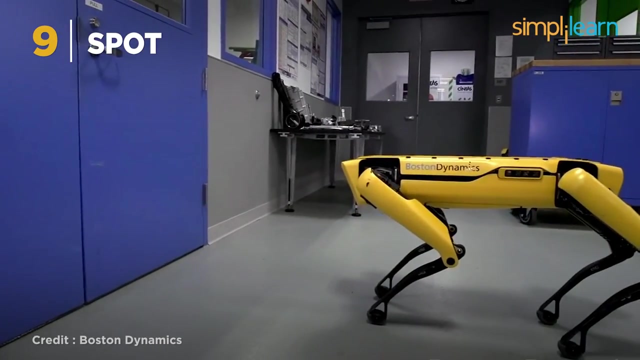 A very important feature of AIBO is that it has an app that owners can use to alter system settings or add new tricks and store memories by connecting to the cloud AI system. Next, on number 9,, we have Spot Former. Spot robot, also known as Spot Mini, is really a four-legged robot produced by 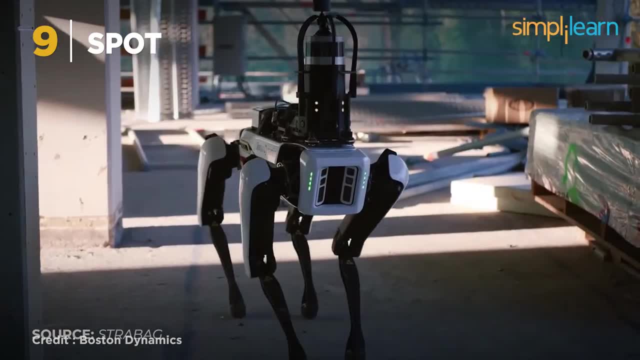 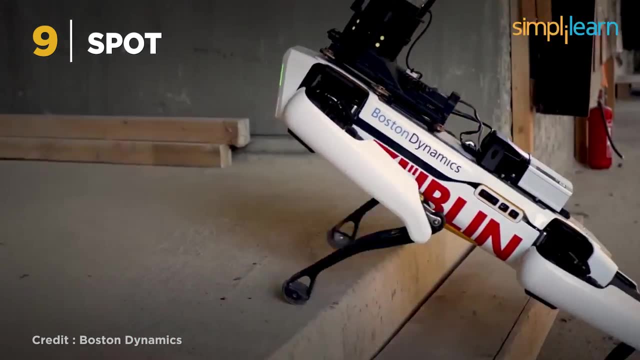 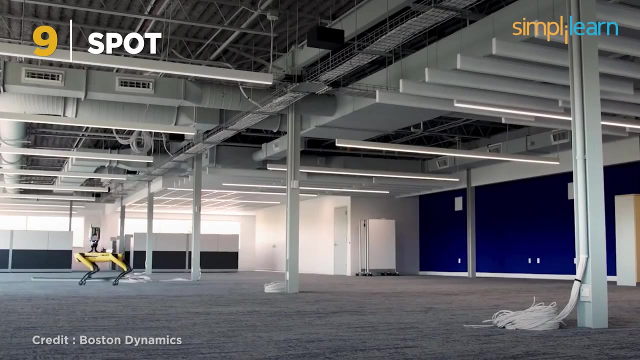 Boston Dynamics, an American robotics company. Spot is 83 centimeters tall and weighs only 25 kg. Spot can perform various tasks, including walking stairs and navigating rugged terrain. It's small enough to be used indoors as well. Spot's unique selling point is that it can go places. 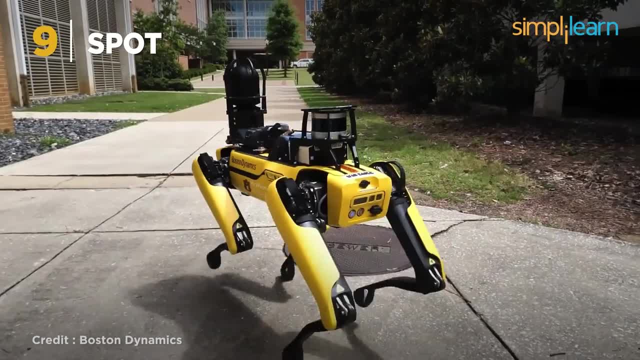 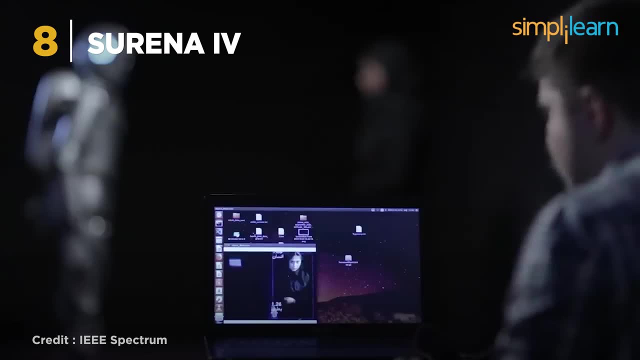 other wheeled robots cannot, all while carrying cargoes of up to 14 kilogram of examination gear. At number 8 we have Serena 4.. Serena 4 is a humanoid robot created by scientists at the University of Tehran. The fourth generation of Iran's Serena robot can imitate a human position. 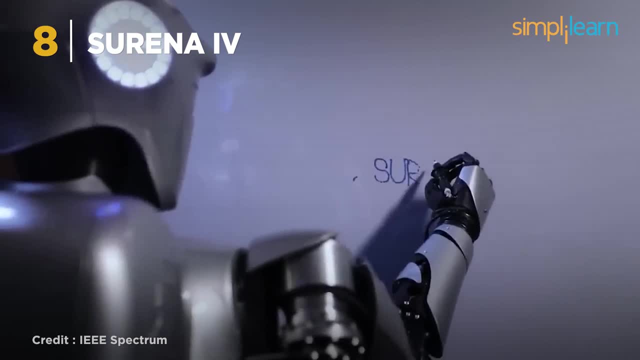 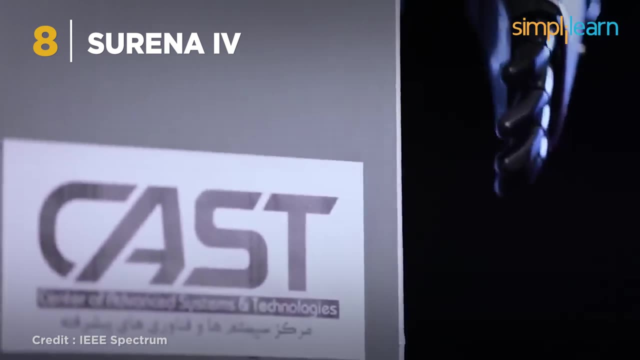 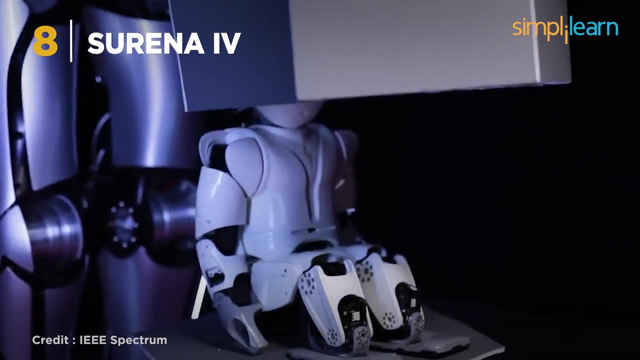 grip a water bottle and write its name on a whiteboard. The robot, which took 4 years to develop, can track objects properly and its new hands permitted to manipulate various objects, from delicate gestures to using power equipment. However, the improvements are not only internal. Serena 4's exterior has been updated with 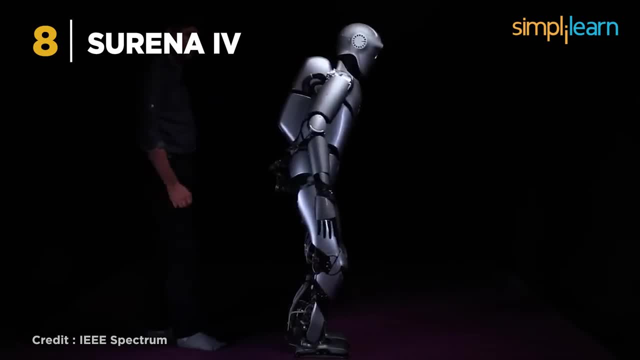 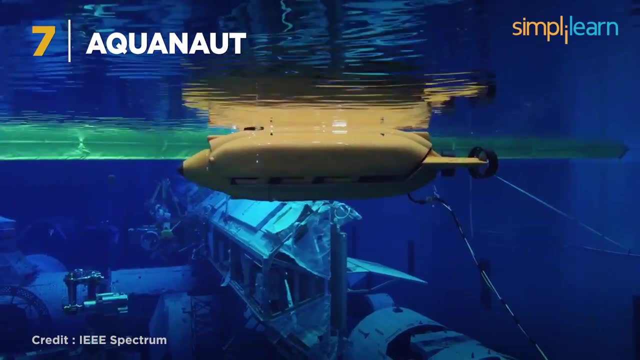 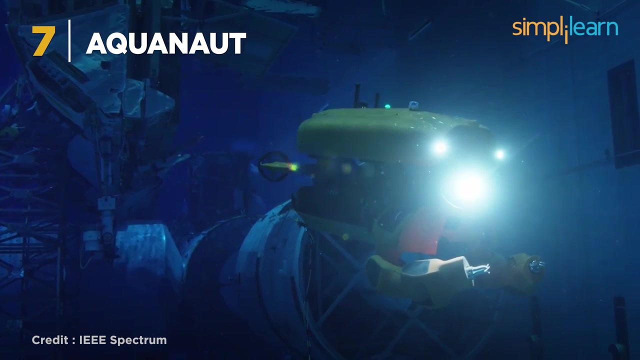 new plastic panels, making the robot appear sleek and just slightly threatening. Next we have Aquanaut at number 7.. Aquanaut is a shape-shifting underwater robot developed by Houston Mechatronics Inc in Texas. The Aquanaut's design allows it to morph from a sleek and small submarine to a slightly 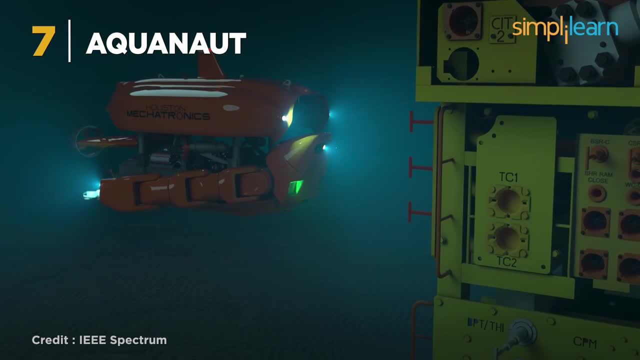 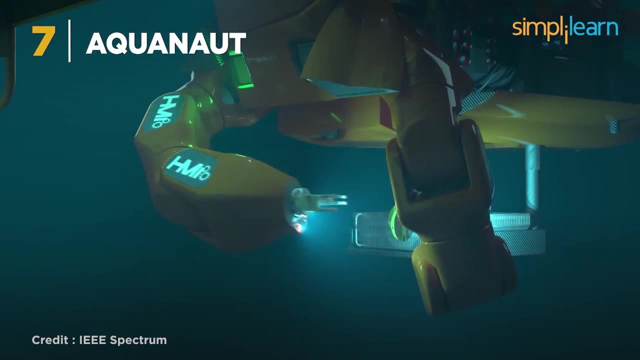 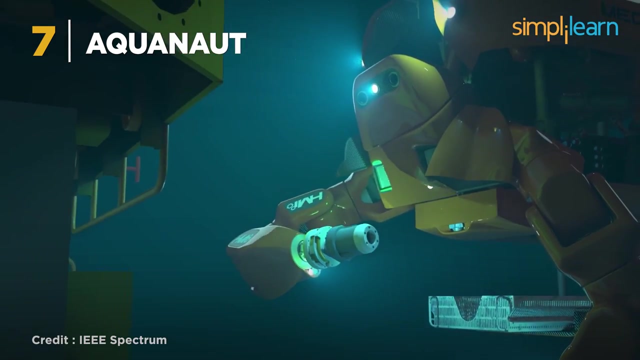 humanoid form with two extended arms allowing it to perform various jobs underwater. Aquanaut was created to address a long-standing problem in offshore oil and gas, which was the cause of maintaining offshore sites. With no similar device on the market, the Aquanaut might have a significant advantage. 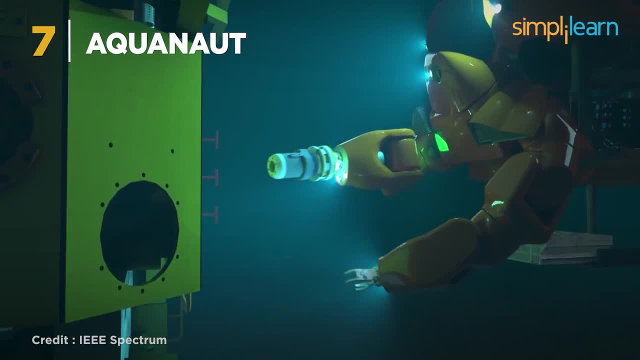 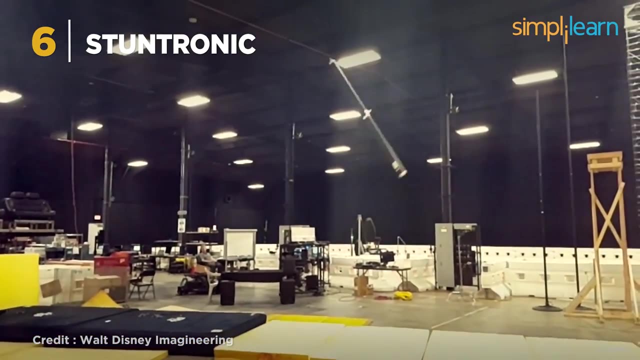 because it can accomplish this task with ease, Without the inconvenience of being tied to a support vehicle and with only minimal oversight from a human operator. At number 6 we have Stuntronic. Stuntronics are simple animatronic stunt doubles. 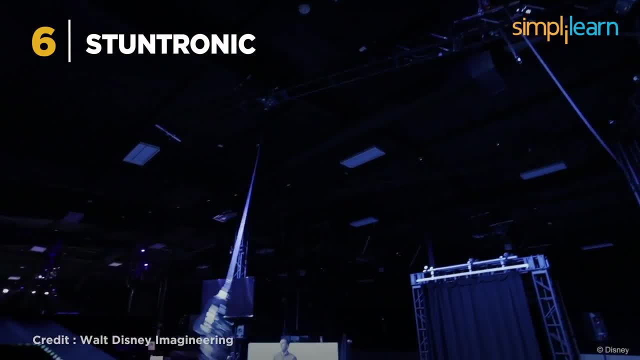 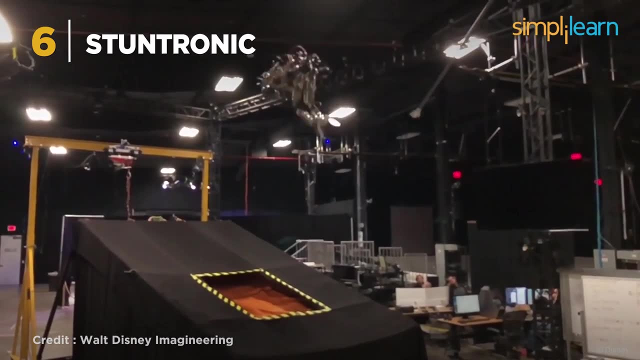 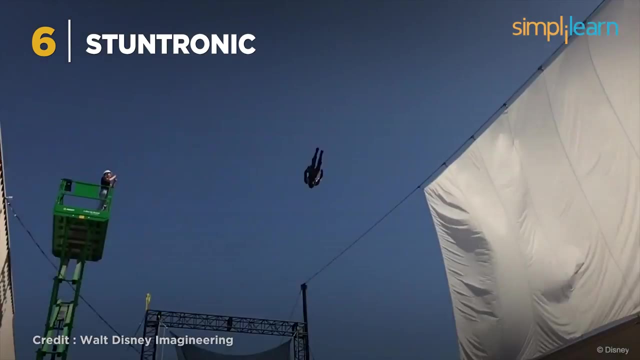 Each stuntronic employs onboard sensing to perform numerous flips, twists and postures with repeatability and precision, combining modern robotic technology with the investigation of untethered dynamic movement. The initiative to investigate stunt double animatronics began with an attempt to manage 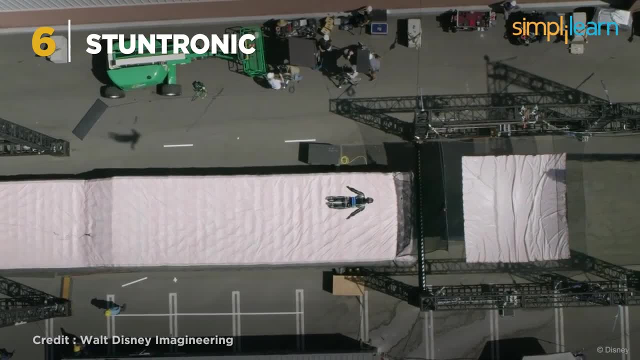 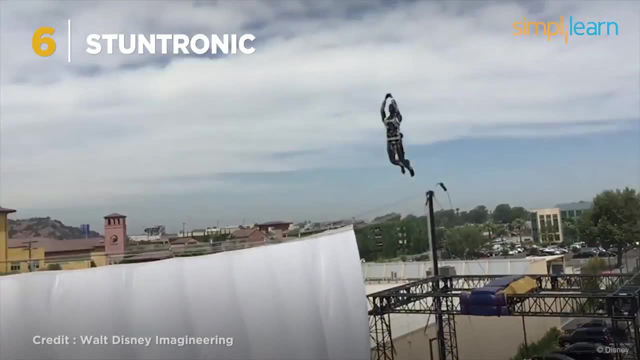 the landing of a figure hurled from a window by Walt Disney Studios. Meanwhile, Disney research experts worked hard to utilize angular momentum conservation to enable fine airborne motion control. A union of the two projects allowed the team to construct the Stuntronics platform, which 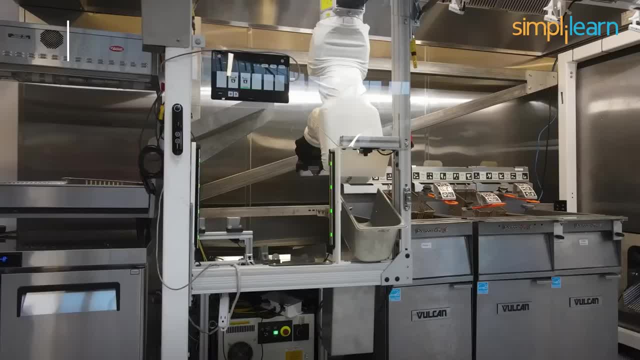 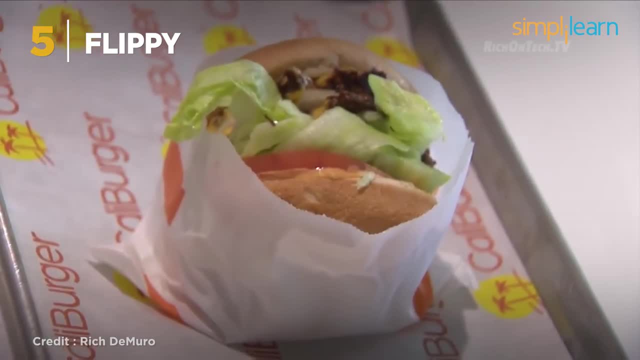 is ready to bring a wide range of dynamic characters to life. At number 5 we have Flippy. Flippy is an autonomous robotic kitchen assistant that can assist chefs in preparing freshly cooked burgers and fried foods such as crispy chips. Flippy is an autonomous robotic kitchen assistant that can assist chefs in preparing freshly cooked burgers and fried foods such as crispy chips. 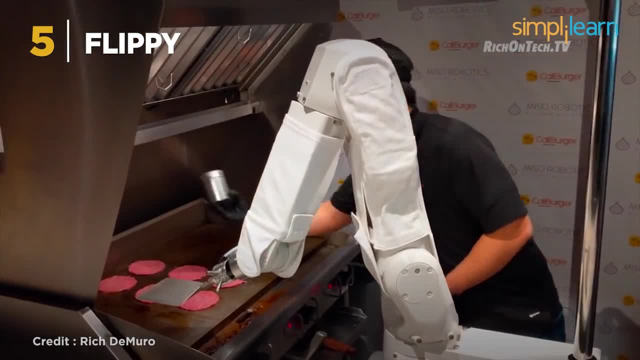 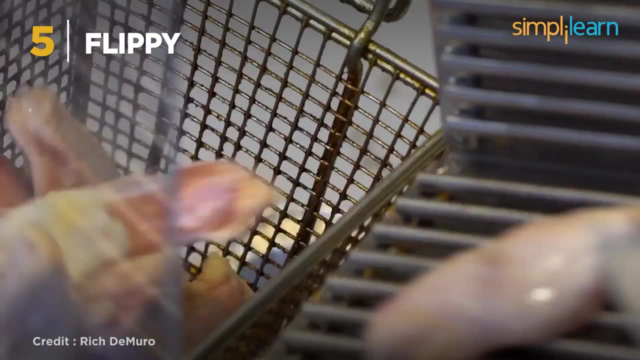 For example, while cooking at the grill, it can automatically detect when raw burger patties are placed, monitor each patty in real time and switch between spatulas for raw and cooked meat. Flippy's brain is powered by cloud connected artificial intelligence, allowing it to learn. 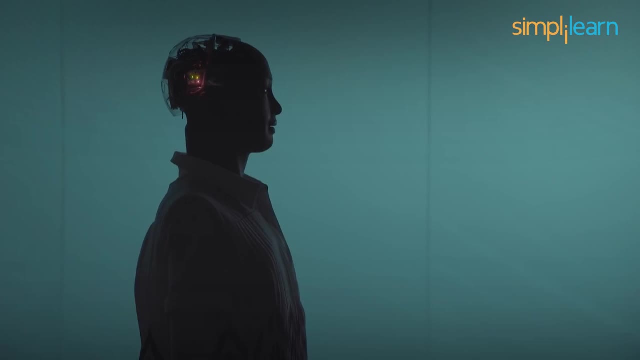 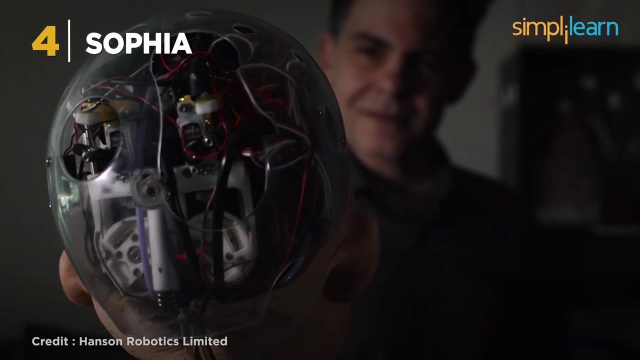 from its environment and acquire new abilities over time. Next, we have Sophia at number 4.. Sophia is regarded to be the most intelligent humanoid robot. She made her debut in 2016 and her interaction with humans from giant mission reel that emerged as an anticipated success and in the music video, Sophia's, of courseает the least concern. 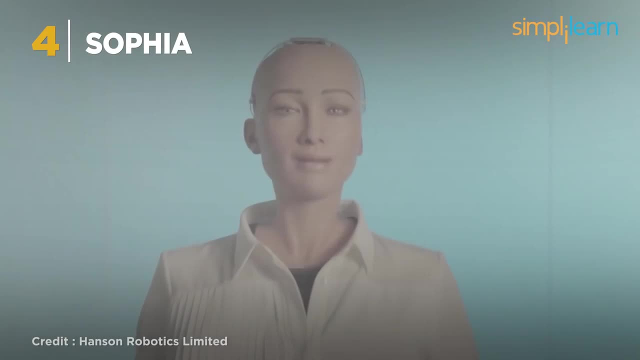 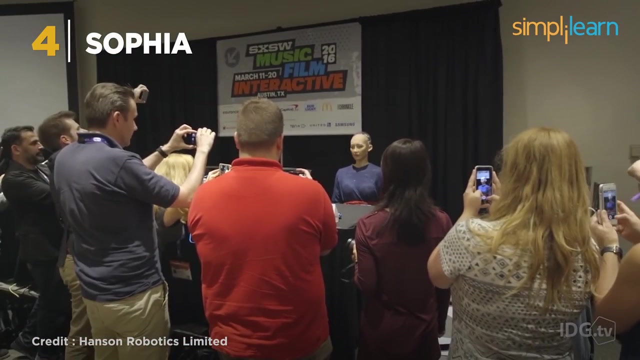 humans was the most extraordinary thing you'd ever witness in a machine. Hanson Robotics, based in Hong Kong, developed her to integrate as an elderly companion in healthcare facilities or crowd management at events. Sophia is the world's first robot citizen and the UN Development Program's first Robot. 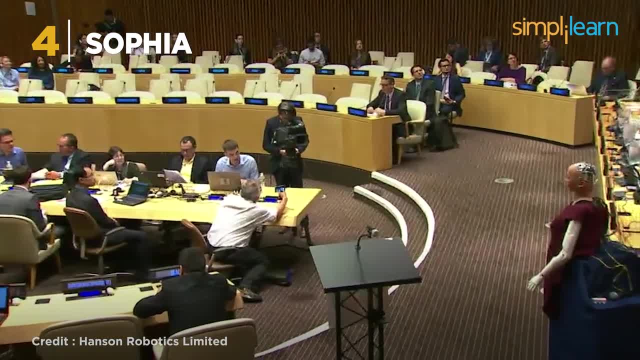 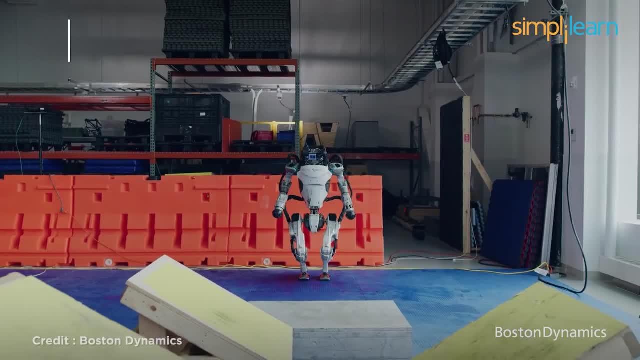 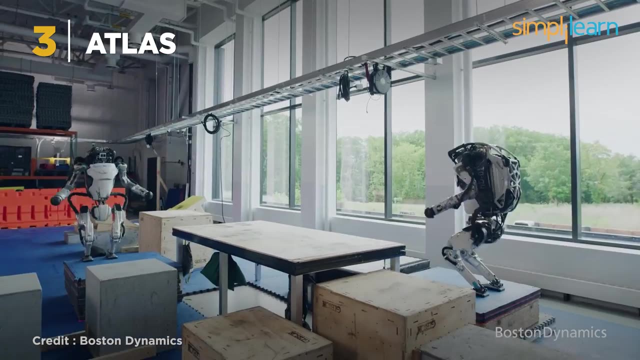 Innovation Ambassador Sophia has integrated neural network models and artificial intelligence to recognize human faces and interpret their gestures and emotions. At number 3, we have Atlas. Atlas is a humanoid robot created by Boston Dynamics and renounced for its unmatched ability to jump over obstacles. do backflips and dance. 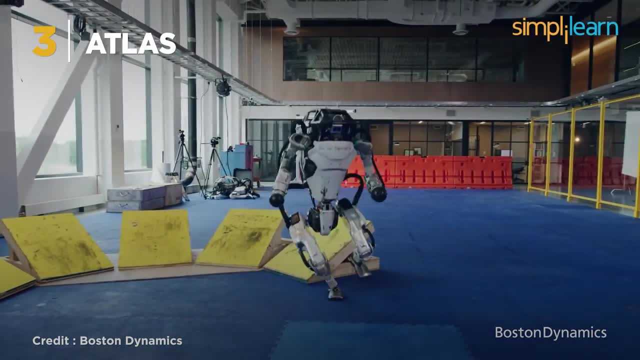 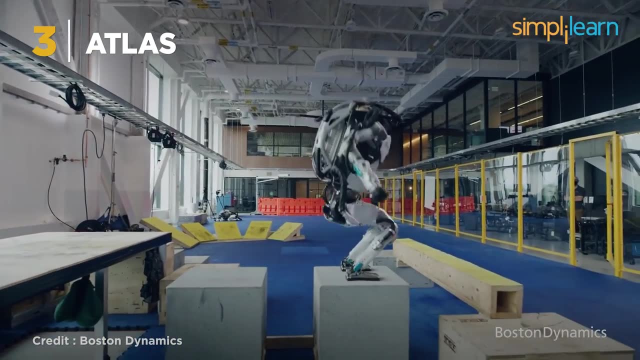 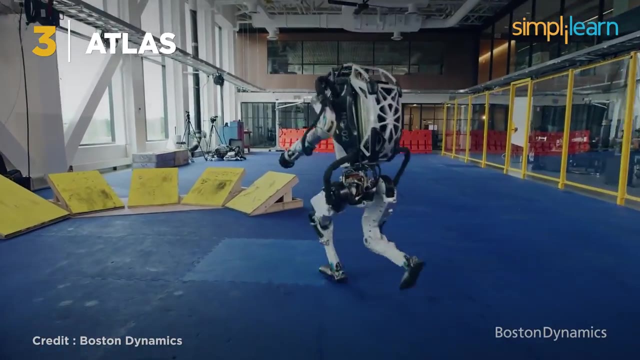 Atlas completes a parkour track in one of the company's most recent videos. Its evolution has been nothing short of remarkable. Aside from the spectacular acrobatics, it demonstrates some interesting foundational abilities, such as awkwardly shifting its equilibrium after landing. Atlas' behavior has also been extended by providing it with a collection of template. 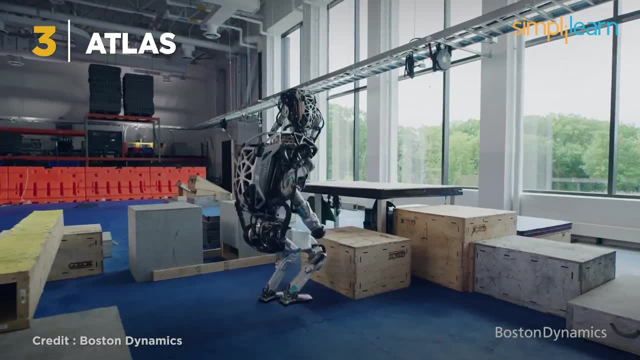 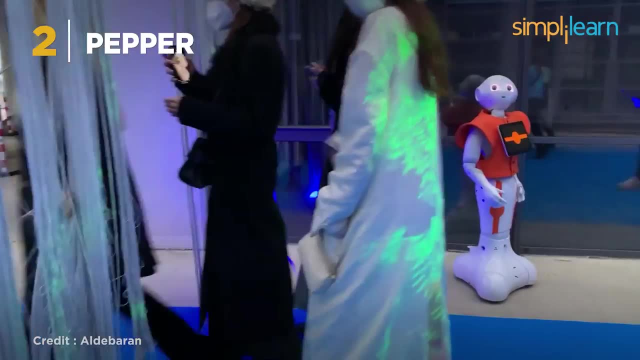 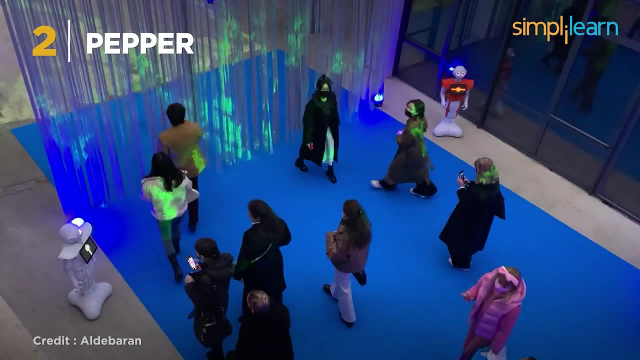 behaviors such as leaping and vaulting, And allowing it to adapt those behaviors to the new scenarios it finds. Next we have Pepper, in the second position. The Pepper Robot is among business's most sophisticatedly commercially available social robots today. SoftPak Robotics designed it to be friendly and engaging, as well as to put people at ease. 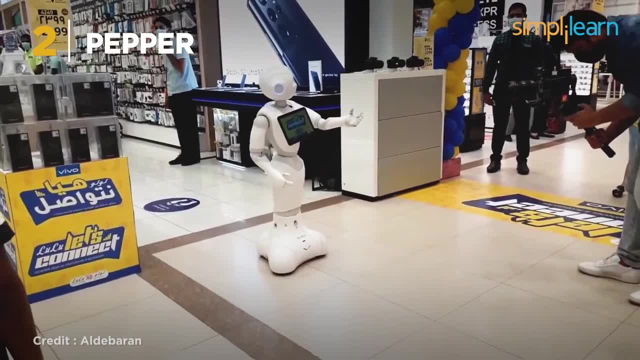 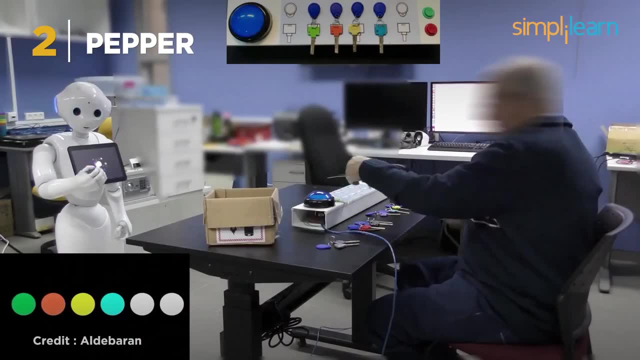 and is equally at home with infants as it is with adults. Pepper can hold conversations and incorporate knowledge from those talks into his words. It may be trained to recognize items, pick them out in a room and may even be able to communicate with others. 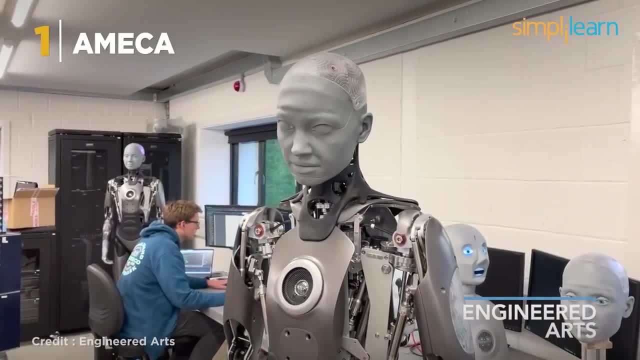 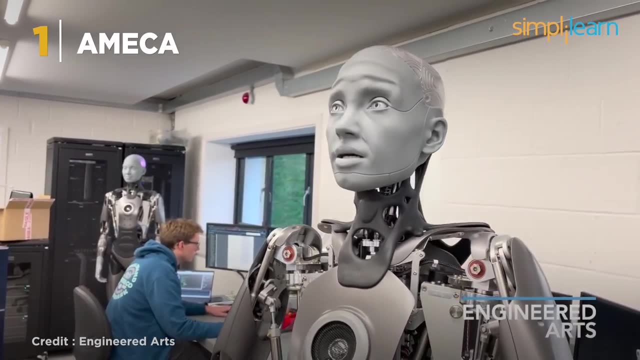 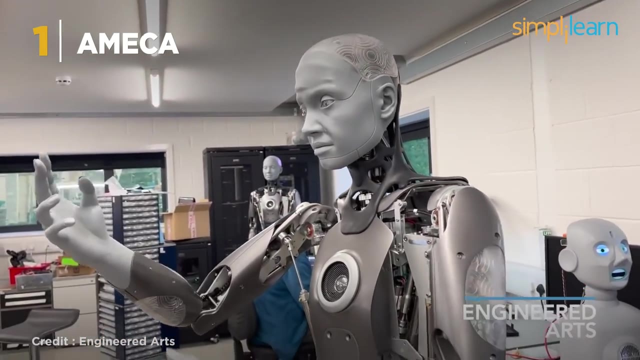 Finally, at number 1, we have Amica. Engineered Arts describes Amica as the world's most advanced human-shaped robot, reflecting the cutting edge of human robotics technology. The robot can mimic expressions fairly well and responds to all questions articulately. 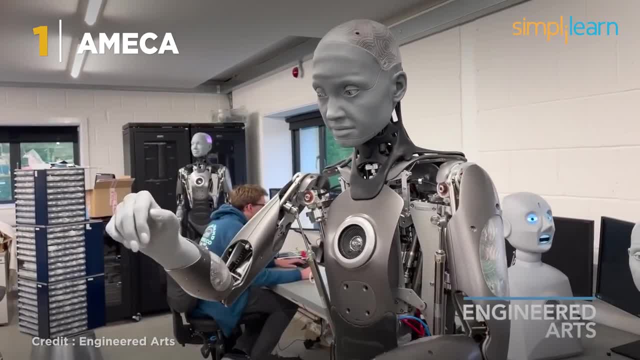 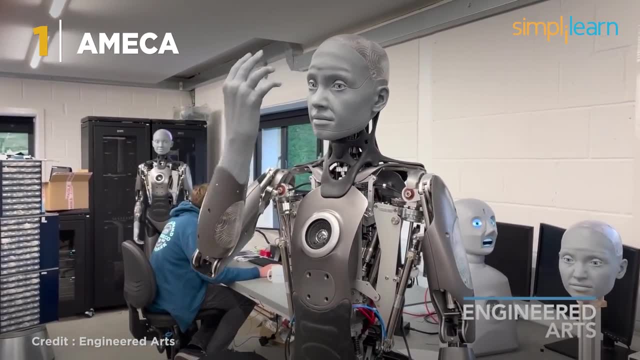 Engineered Arts' Amica hardware is based on the research into humanoid robotics and is built on their proprietary Mesmer technology. Amica's artificial limbs, ligaments, motors and sensor arrays are made with the help of cutting edge technology. As shown in movies, the rise of AI usually results in chaos.